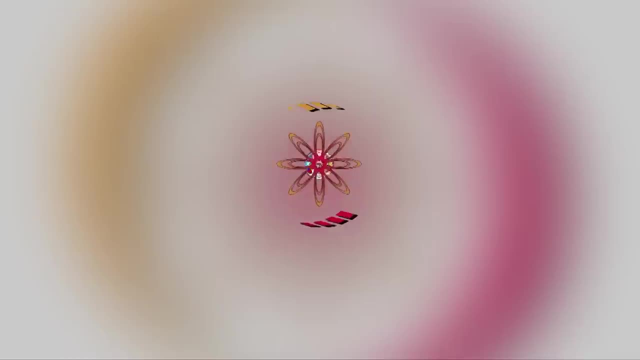 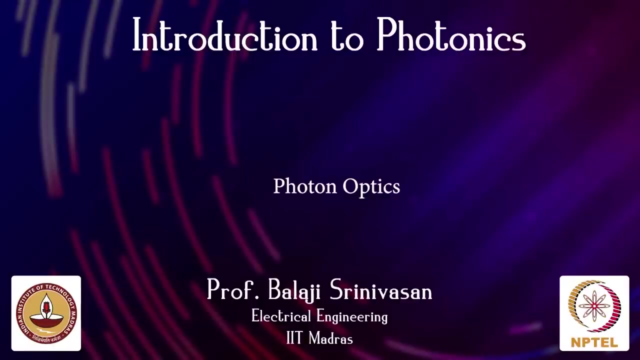 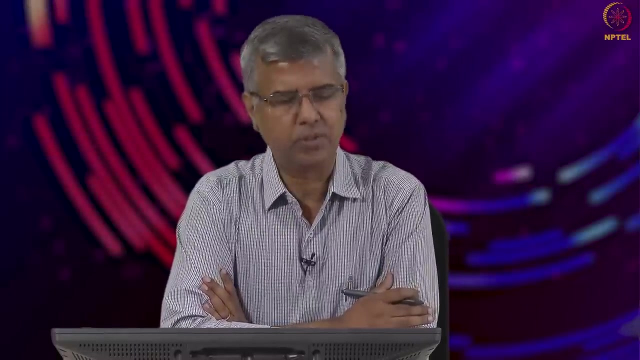 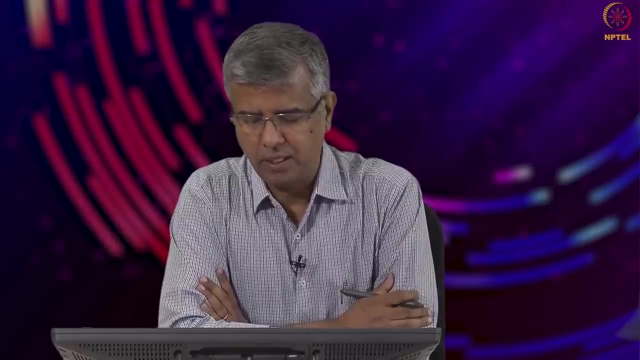 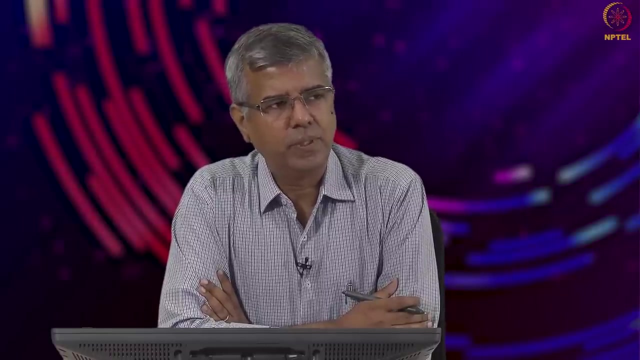 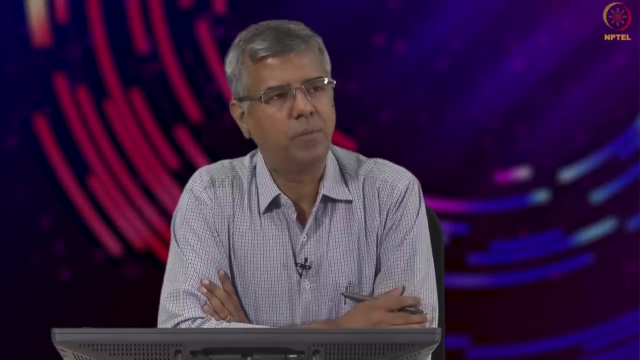 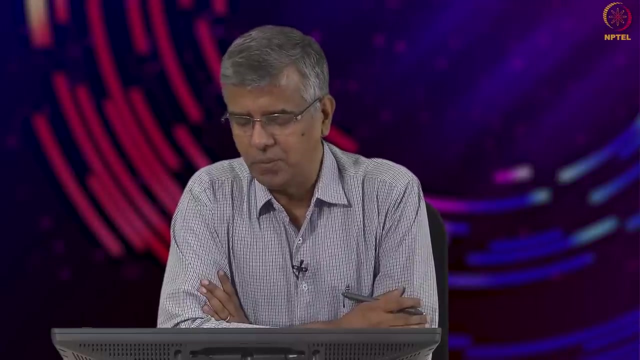 Good morning, welcome to Introduction to Photonics. We started last week with the learning outcome of identifying fundamental principles of photon optics and quantifying photon properties. Since this picture is drastically different from the kind of things that we have been seeing previously, just from coming from the particle nature of light, we had been spending 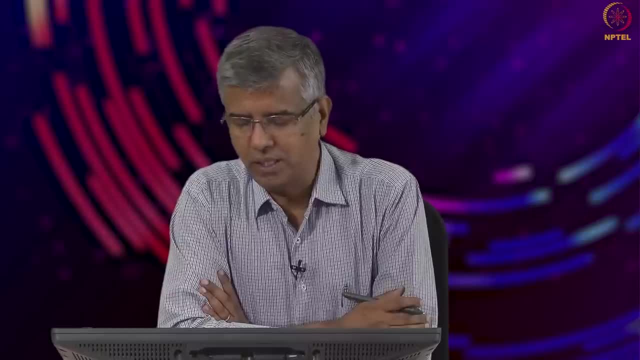 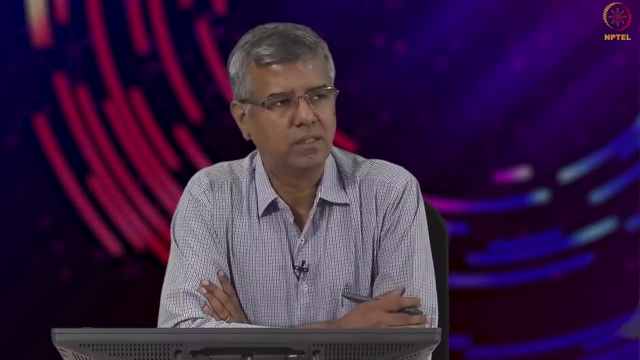 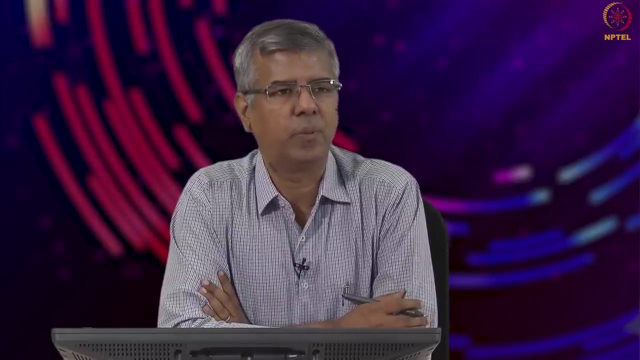 a little bit of time understanding what this means and, of course, one thing that helps in this: understanding that these photons, in one way of looking at them as particles, but they do exhibit wave nature, So they have a wave particle duality and through that duality, 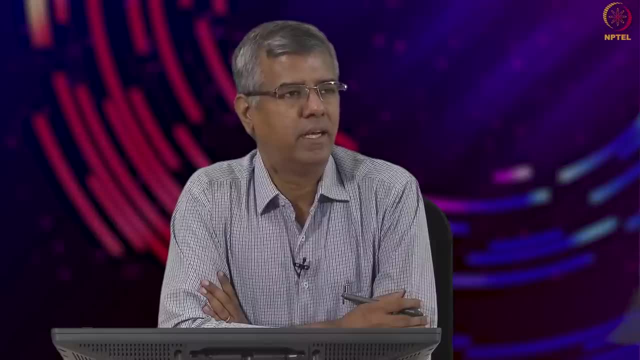 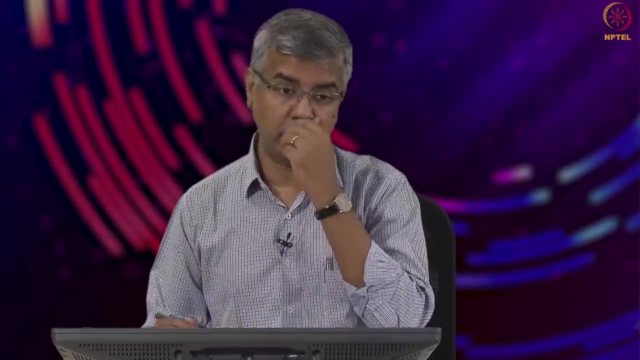 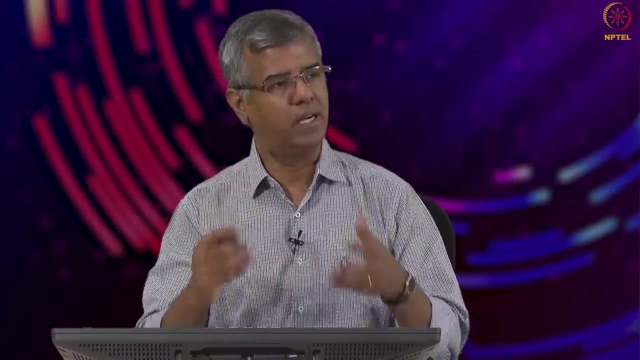 we can bridge across and understand a lot of properties from the wave picture as well. right, It gives us an opportunity, But, trust me, what this picture also allows is To get a little more insight which cannot actually be explained so well using the wave. 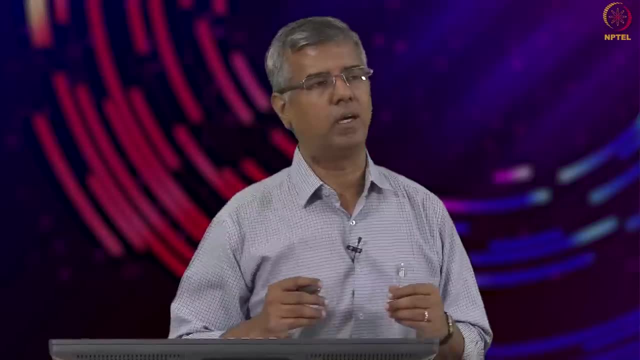 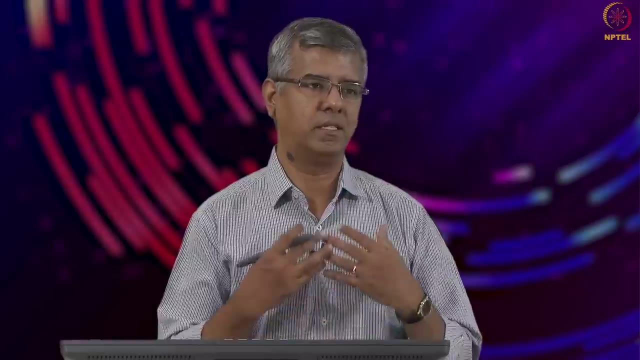 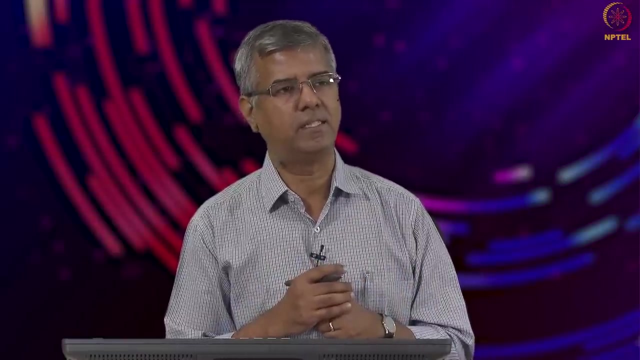 picture, and that is what we are getting into. in the next few weeks, We will talk about light emission and detection, which, as we will understand, is a quantum phenomena. right, There is a certain quantized interaction that is happening, and that is what we will read. 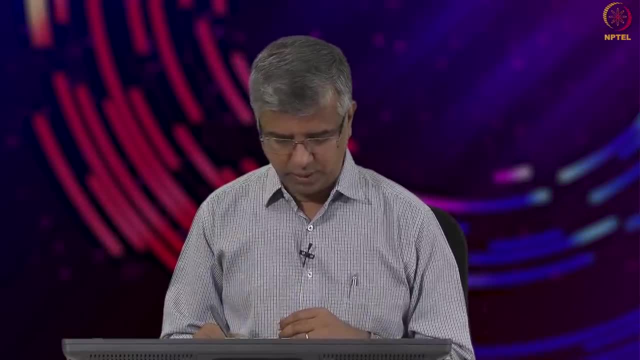 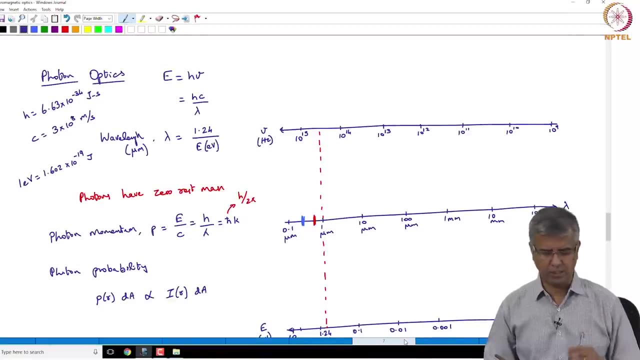 about Now before we go on. I just wanted to clarify one particular thing. of course we talked about, you know, when, in the photon picture that the you know define an energy of a photon which corresponds to the frequency, and we were looking at that relationship. We will look into that a. 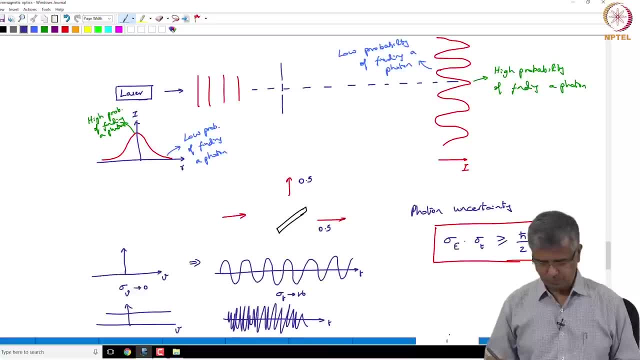 little more detail today, But before. So before we go on, I wanted to actually clarify something, and this was actually something that was pointed out towards the end of or after the last session, So somebody was pointing out this part is very clear that you know we have a monochromatic 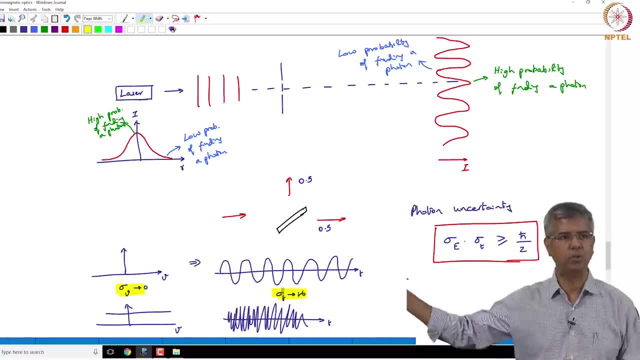 wave and to characterize that monochromaticity you have to observe for infinite time. But the converse was not as clear, was the specific comment. So to essentially clarify that, let us just take a very short pulse. so the pulse is such that your, You know, your- uncertainty goes to 0, tends to 0, when would the uncertainty tend to 0?? 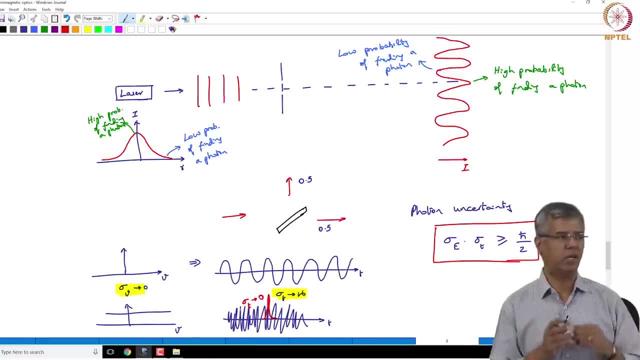 When you have a extremely short pulse within which all your photon energy is present. right, If you have an extremely short pulse, what we find is that, you know, through the inverse Fourier transform, You can Rather through the Fourier transform, you can find that it actually corresponds to a large 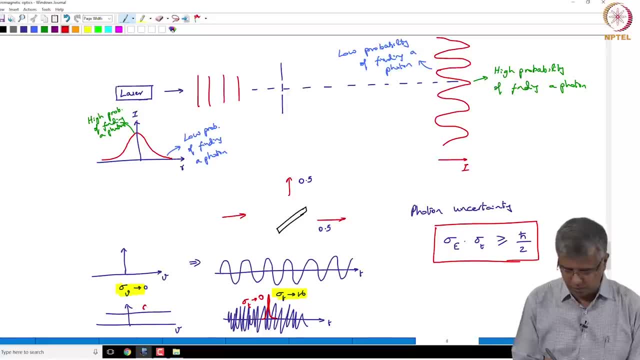 range of frequencies. So that is what we are talking about here. So this uncertainty in frequency actually becomes infinity, because we are representing- by going for the short pulse, we are representing a very large spectrum, Ok, You know, a very large range of frequencies. 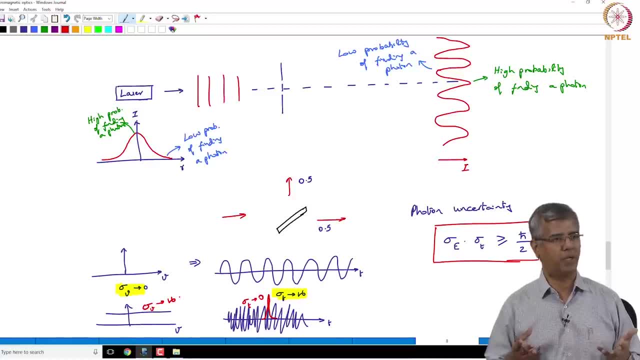 So that is the reason we are talking about the spectral band. So give you an example: if you take a femtosecond pulse- you know people have actually demonstrated at a second hundreds of attosecond pulses- you can believe that right, But if you take a femtosecond pulse, that typically corresponds to a spectral width of 10 power. 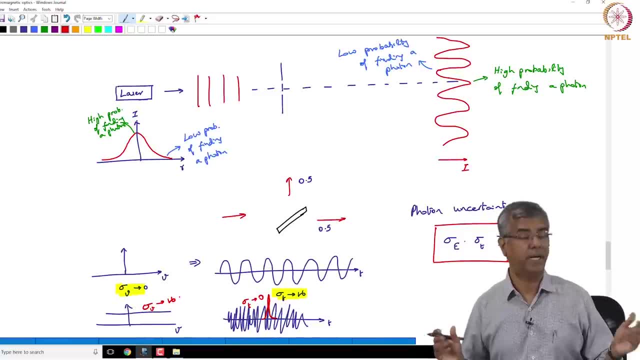 15 Hertz Right, So that is actually a fairly large range of frequencies. And then there is also a spectral width of 10 power, 15 Hertz Right, and so you can essentially say: shorter the pulse, more will be the spread in frequency or more will. 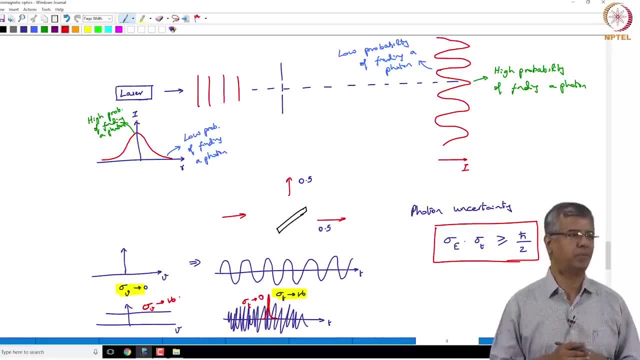 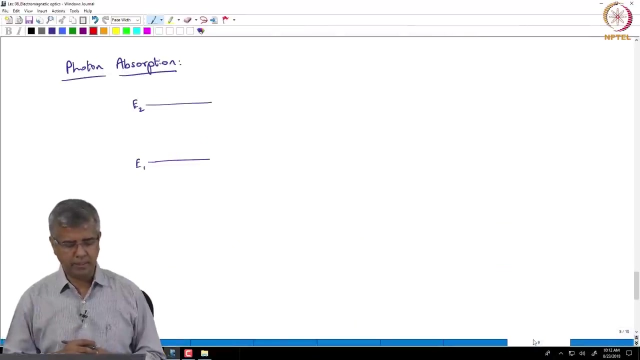 be the uncertainty in determining a particular frequency, associating a particular frequency to this, to this light pulse. right? So that is the converse picture. ok, So that was just a clarification from the previous lecture, But let us just go on to this other topic. 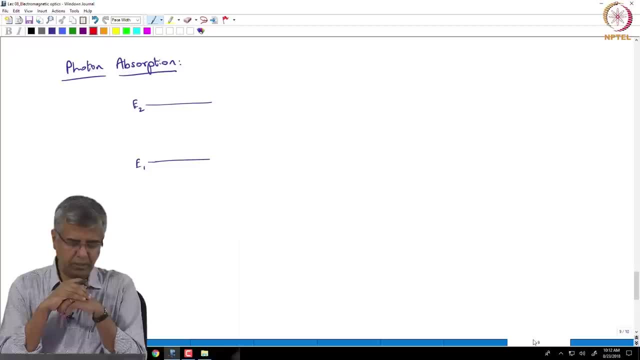 photon absorption. I am actually considering this topic. one side is to project the utility of considering an energy of a photon, ok, but the other side of it is also that you know, you got to know the voltage inte stellt energy. you got to know the battery moment f upon in 음. 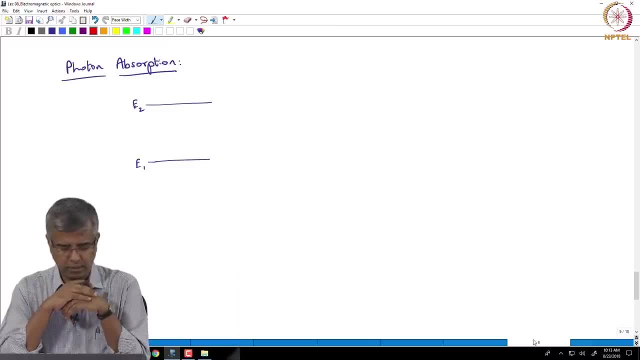 going to be a demonstration that is going to be done this week, So let us see how light absorption happens. So if you have two quantized energy levels and these energy levels, mind, you could correspond to two orbitals of an atom. right in an atom you have all these electrons orbiting. 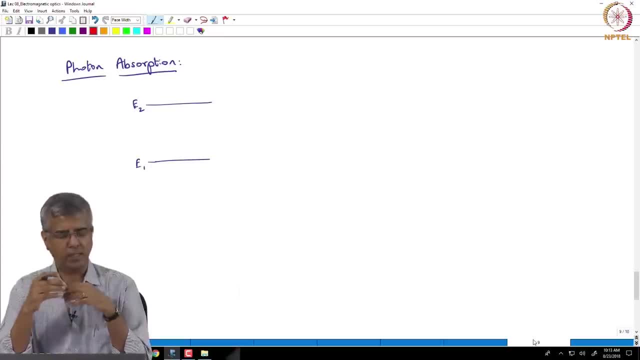 the nucleus right. So these could be two orbitals. let us say the lower energy level corresponds to the valence orbital and a higher energy level corresponds to, you know, a higher orbital. higher energy level corresponds to the valence orbital, Outer orbital, which normally is not populated. there are no electrons in that, because all your 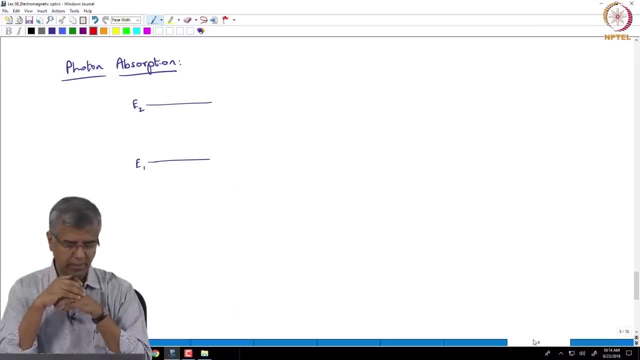 valence electrons are at the lower energy level, right? So in this case, what kind of light can you possibly absorb with this atom? Can you absorb any frequency of light? Yes, No right, you can absorb only a specific frequency which takes the electron from. 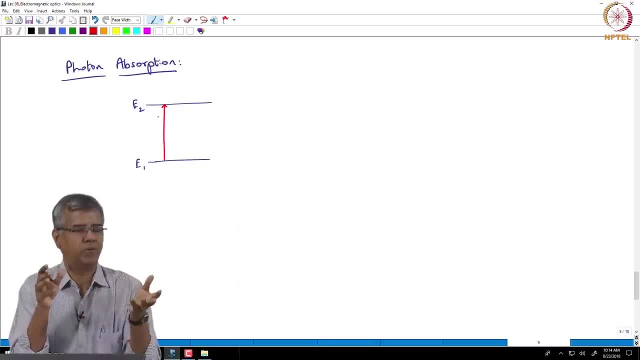 one orbital to another orbital. all the other orbitals are forbidden, right as far as this atomic system is concerned. So this will happen only if you have an energy of a photon which corresponds to delta E, where delta E corresponds to the energy difference, right? 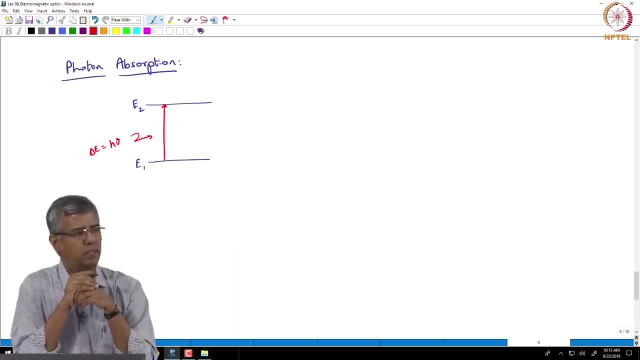 So in this case you will have the absorption happen. Now, if you are considering absorption in the collection of atoms, right, you are normally not either in the collection of atoms or at the absorption of the different particles. right, isolating one atom and looking at the absorption. but you are looking at a collection of atoms. 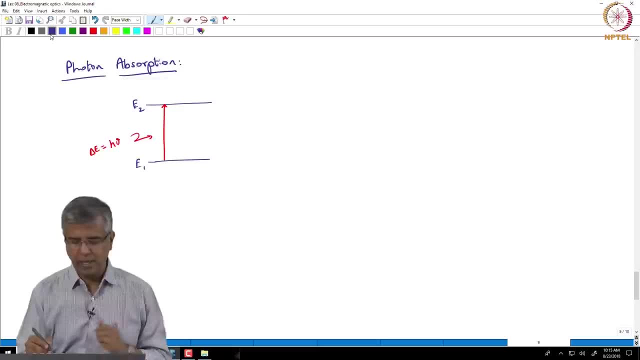 When you are looking at a collection of atoms, you may have this higher energy level is may not be one energy level and the lower energy level, that specific energy level or the specific orbital position may be different at different sites. or you could also have this situation where, when you 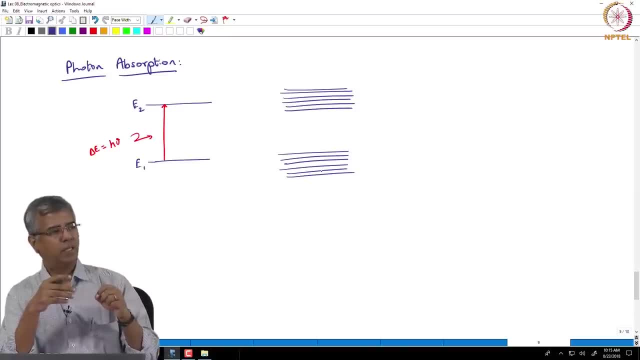 have collection of atoms, they end up splitting that orbital. there is something called stark splitting that happens, which allows you to go from one energy level to a collection of energy levels. Ok, so when you consider A collection of energy levels, what does this represent? now You have a possibility that you. 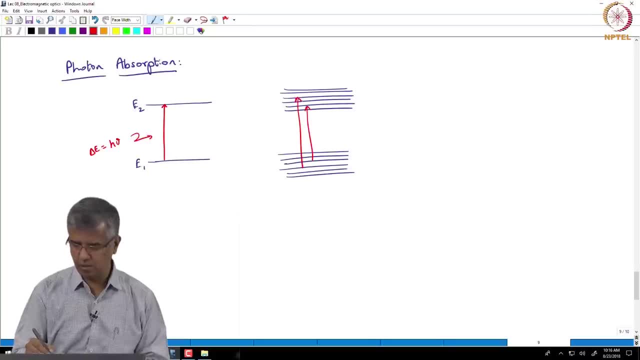 could get absorption over a wide range of transitions. So, in effect, when I am looking at absorption over a wide range of transitions, So, in effect, when I am looking at absorption As a function of wavelength- ok, in this case it would have been a delta function- is only one. 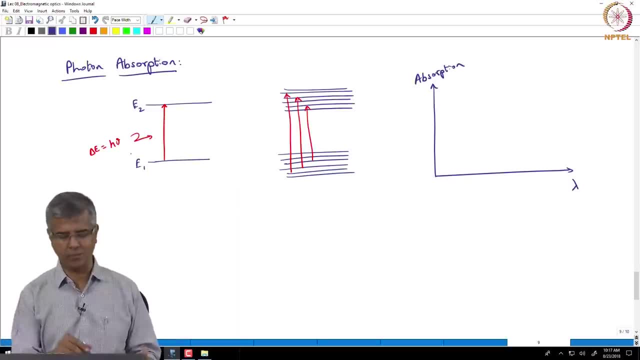 particular frequency or one particular wavelength, that can get absorbed in a isolated atom case, Right, but when you are looking at a collection of atoms, you can. actually you have a band, a spectral band, over which the absorption can happen. And this is actually going a little more detail. we will actually come 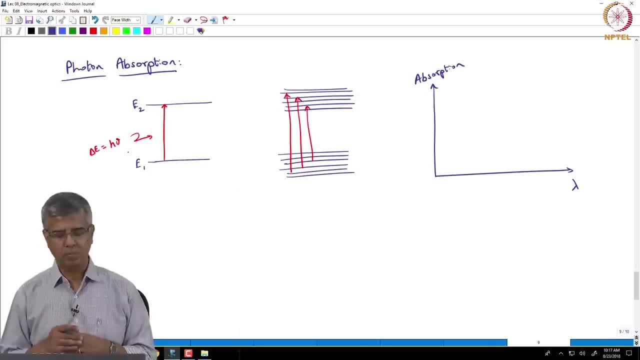 back to this at a later point. but the point here is that all these transitions are not equal probability right. If they were equally probable right, the absorption would have extended from one frequency to another frequency and absorption would have been constant across that entire. 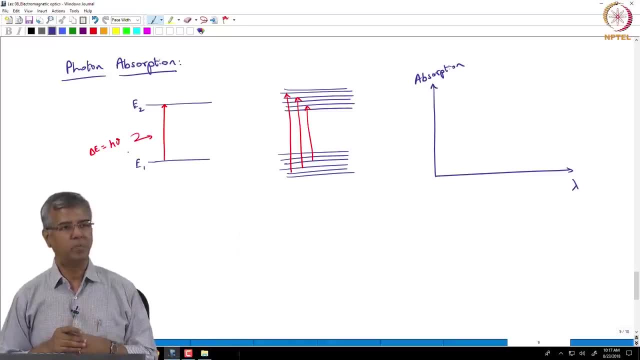 spectral band, ok, But there are some selection rules that come into the picture, that it actually goes into the quantum mechanics of this, And you talk in terms of, only in terms of probability of absorption, and it so happens that this absorption would now- well, I will use blue. ok, So would 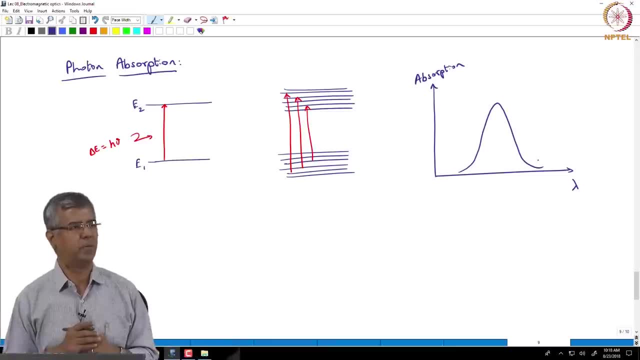 be over would be spread over a bunch of frequencies. ok, So whenever this absorption happens and an electron jumps from one energy level to the higher energy level, ok, at the higher energy level it is not allowed to, you know, stay forever. This means the absorption happens in the end. However, way of 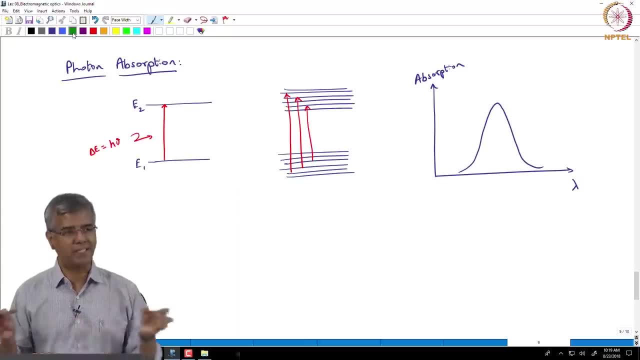 absorption is called instant ontology. Yeah right, the absorber of electrons can be suppressed with any right because the valence energy level is not filled, So it is the higher energy level is what is called a metastable state. it goes up there, spend some time and then comes back. ok, 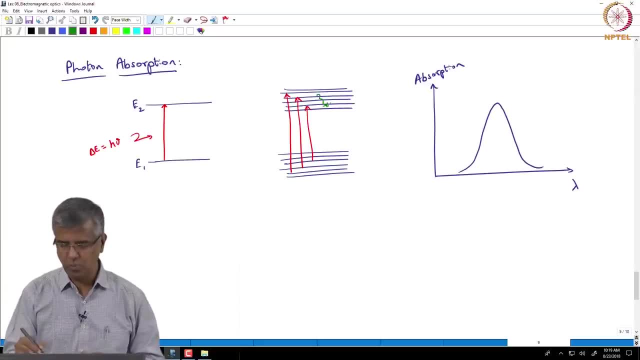 So in that process you might have some non-radiative relaxation happening. right, that is actually. it may lose some energy and then it would go through this emission. And, mind you, when it goes through an emission process, two things to note: it is always from one energy level to another energy level. So 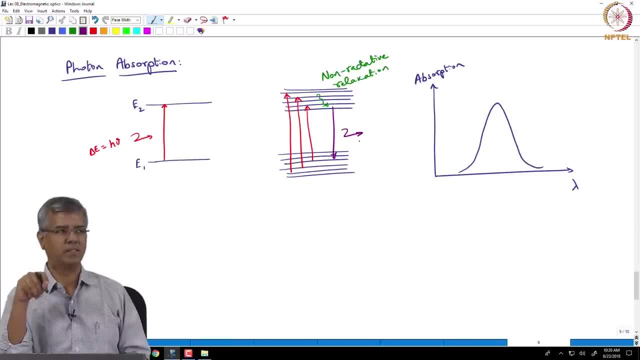 what do you expect when that emission happens? The emission will be quantized, and that quantized emission is what we are calling as a photon with a very specific energy. So let us say the absorption is characterized as h, nu, nu, x corresponding to the excitation. and now 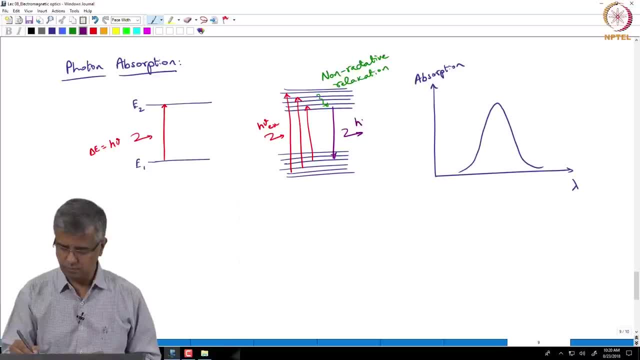 what we are saying is corresponding to the emission. you have h nu emission right And since there is certain energy that is lost and that energy loss could happen above, or it could happen below, also in the ground level manifold, Since that energy loss happens, you can basically say: 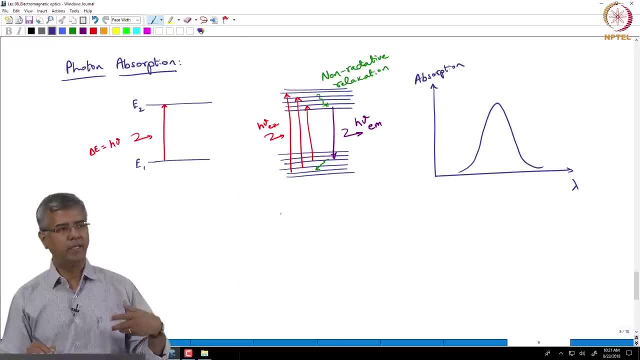 that typically the excitation frequency or the excitation energy is going to be larger than the emission energy. you lose certain energy in the process and you can also say that the excitation frequency is going to be greater than the emission frequency. So if my absorption is happening in this broad 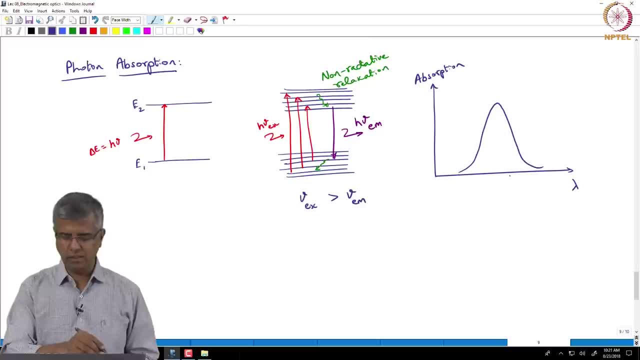 spectrum. how do you think is your emission going to look like? That will be shift to longer wavelengths because you lose certain energy in the process. and you can also say that the longer wavelengths represent lower energy, right? Because in the process of emitting it is losing. 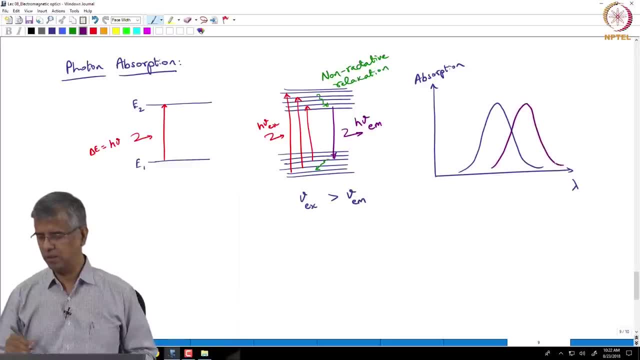 some energy, So your emission would have shifted. okay, Mind you, I have shown some regions where it is overlapping. What does that mean, Since it is actually a broad spectrum? it is actually a broad distribution at the higher energy level and the broad distribution at the lower energy level. You. 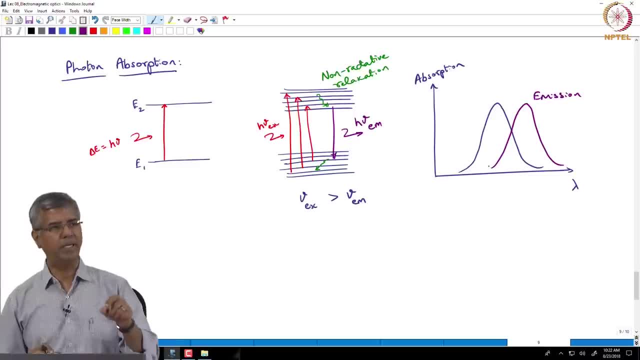 could have a photon that is emitted and you could have, I mean, a photon that is absorbed and a photon emitted. both are, you know, almost having the same energy, right? So this week you are going to see the two different types of radiation here, right? So this is the hydrogen and this is the carbon. 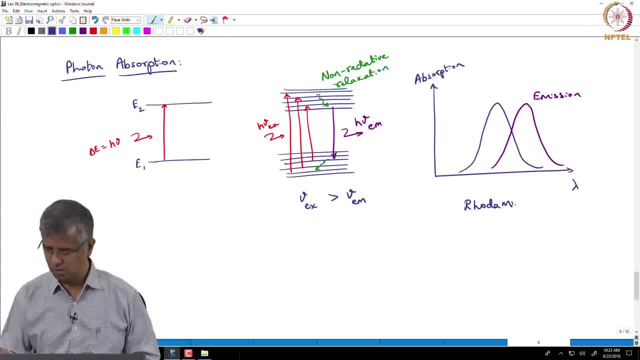 So you will have a basic demonstration of the hydrogen and the carbon. okay, So you will have a demonstration using dye known as rhodamine 6G. so that is a dye molecule. Rhodamine 6G has an absorption spectral band. 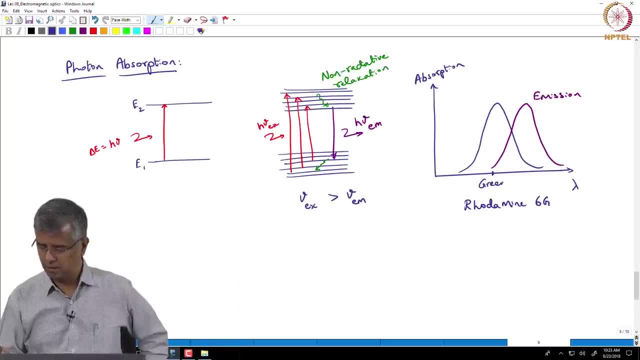 around green and if it is fifth-grade it moves to the upper energy. But you will see if it is fifth-grade or a fourth-grade, then the oxygen is going to stay there. okay, So the oxygen is going to stay there for a long period When you lose the oxygen. 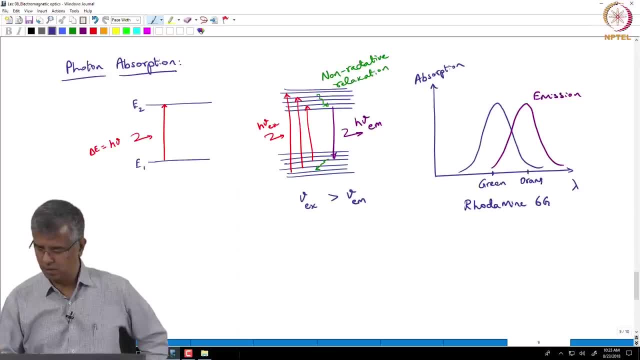 an emission spectral band around orange color. ok, So if you come in with red color into this Rodaman 6G, what do you expect to happen? There would not be any absorption, because red color in this case would correspond to some transition, like this right, which is forbidden, right. So 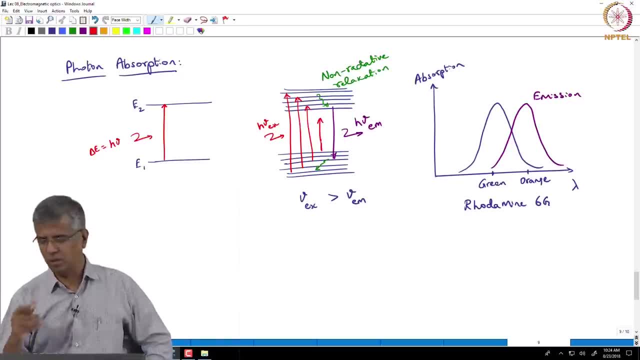 you do not have a corresponding energy level to go to, so, because of that, there would not be any absorption. ok, So this is part of what will be demonstrated to you: that you will come in with red light and you will see that it goes to. 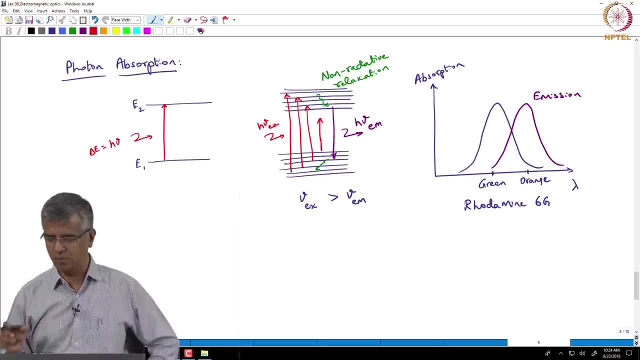 right through this Rodaman 6G solution and if you have green light coming in, it will be strongly absorbed. you will be able to see the absorption. So what do you? what a strong absorption mean? Essentially, if you have more number of these Rodaman 6G molecules, more will be the absorption. 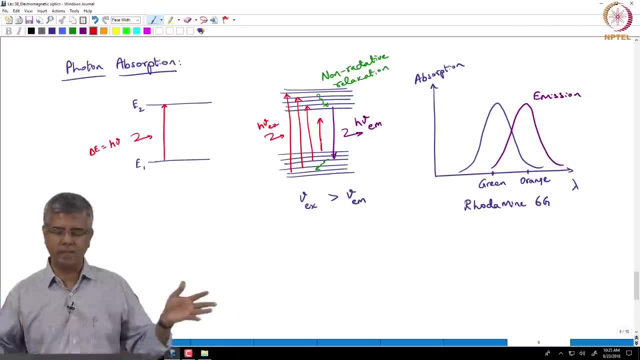 ok, Ok, Right. So you will see that you will be given like three different concentrations and if you are asked to figure out- which is what you know- what are the relative concentrations, you come in with green light right, Hit that solution with, let us say, you put it in a transparent cuvette. so 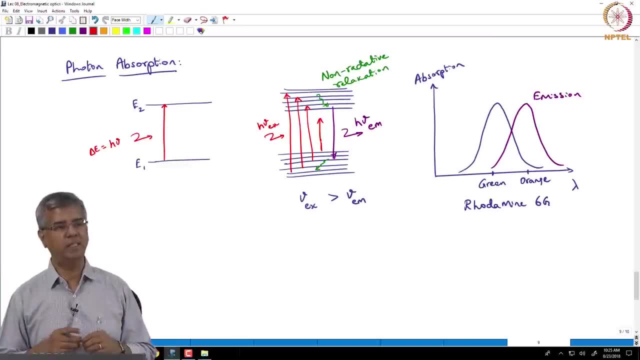 you can see that absorption: with the highest concentration it will all get absorbed within a very narrow region, right, Ok? Whereas with the lower concentration it will be absorbed less drastically, so it will actually, you know, you may be able to see light there. some of that green light come through the other side. 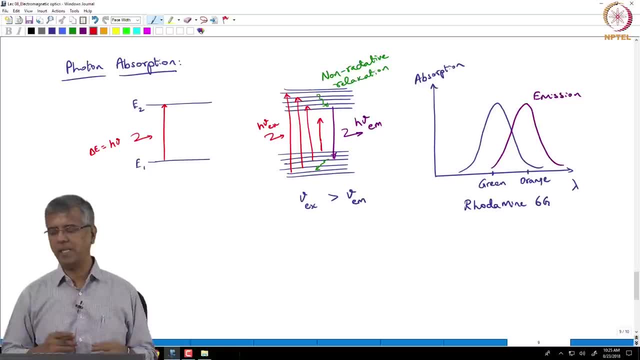 ok, And you will also see that whenever that absorption happens, there is also an emission that is happening, and you will be looking at this orange emission. you will be observing that orange emission, Ok, Ok, Ok. One of the things that we will do as part of that is also use some color filters, and you already seen some color filters, right? What was the? what is the context in which we discuss color filters previously? 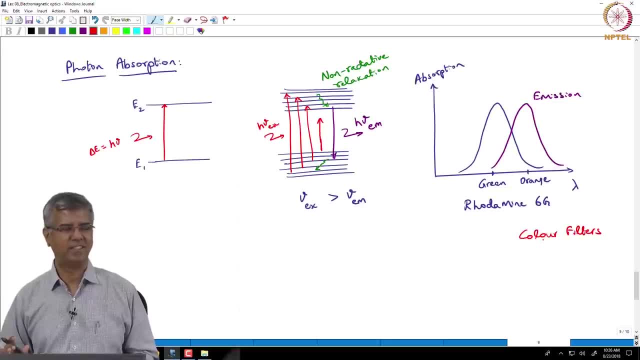 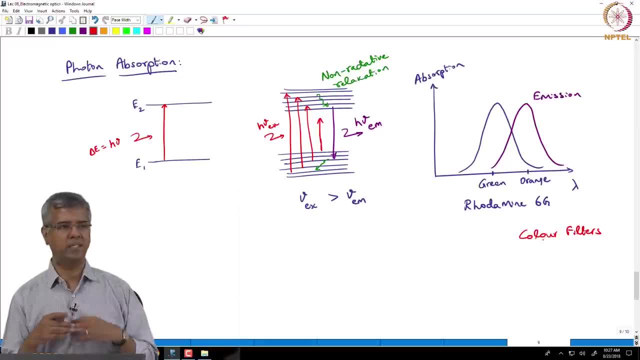 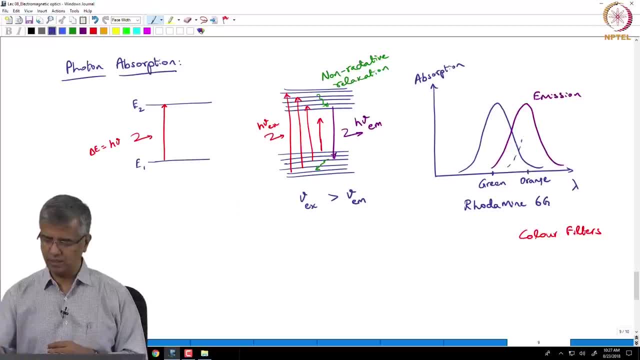 Ok, Ok, the absorption for the other one. if it is some other dye, you know, it may look like that, and then in between those two there is very little absorption happening. So what that means is any color between these two will actually be transmitted, So you could have color filters. 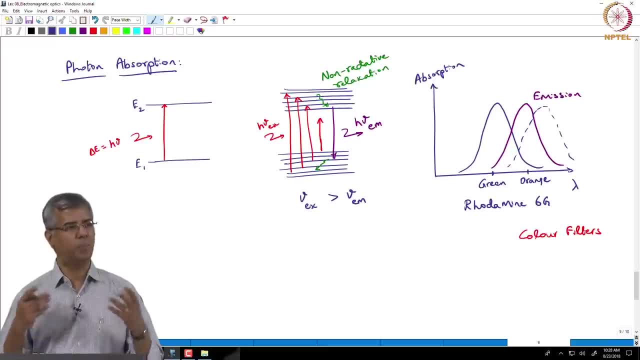 made by doping, a polymer film with my different dye elements, such that you define which areas get which spectral regions get absorbed, which gets transmitted, So you may be able to differentiate colors based on you know the such principles, So you will get to you know work with those color. 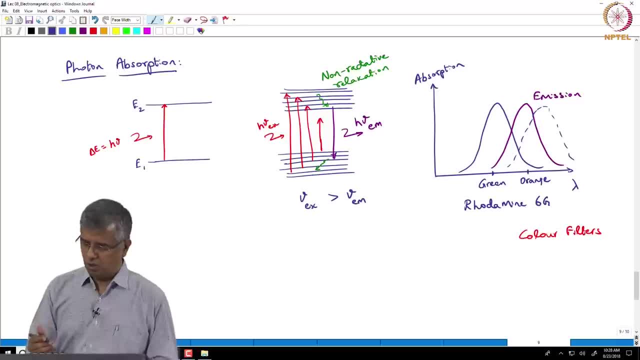 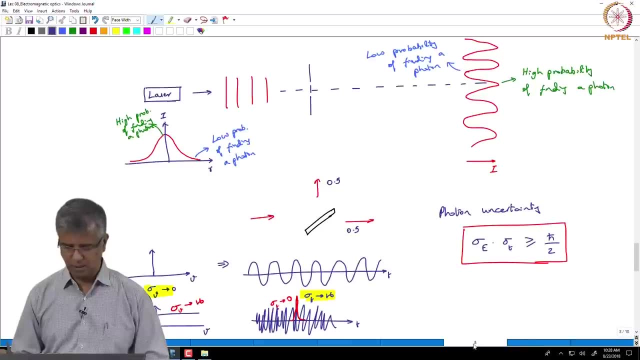 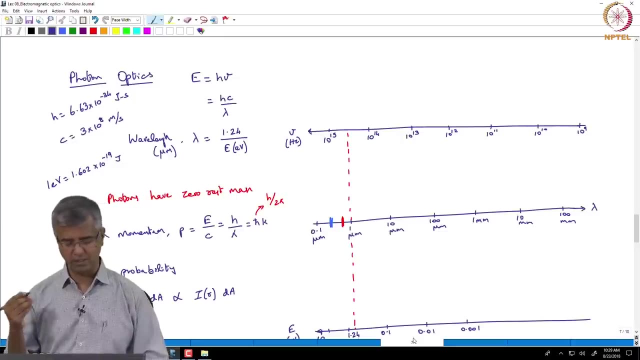 filters and you will be able to do that. Thank you also this week. So when we were considering all the photon properties, so we were talking about that the photon has some energy, has zero rest mass, but it has some finite momentum, a probability of finding a photon, and then we were looking at photon uncertainty. But 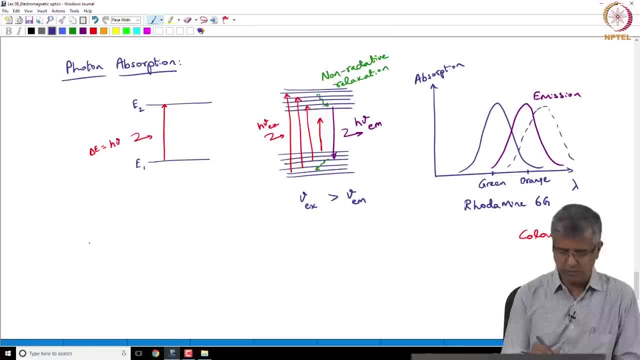 there is one more property to the photon which I would like to address now, which is called photon polarization. So what does photon polarization mean? So you can look at a photon as a particle and if the particle is spinning around its axis, while it is travelling right, It is spinning around this axis, It can. 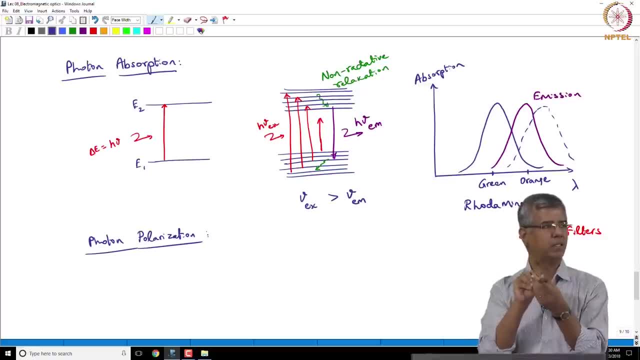 either spin this way or, you know, clockwise or counterclockwise. Those spin could would essentially mean that the electric field corresponding to that is also spinning as it is moving right. So just that spin itself. since it is just a single particle that we are considering, that field would actually correspond to a 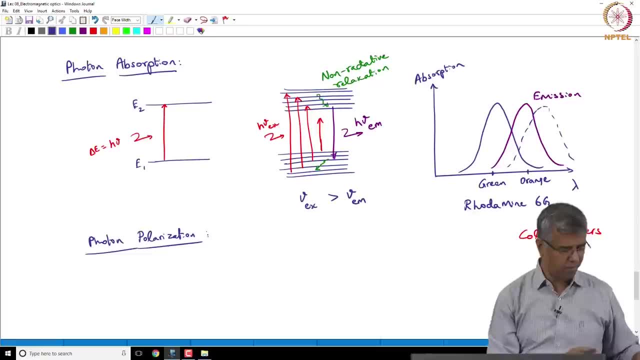 circle. ok, So you could have basically a photon spin which would represent either left circley polarization polarized light or right circley circularly polarized light, depending upon which way it spins right And correspondingly it will have what is called a spin angular momentum, ok, which is defined by S, equals to plus or minus H. 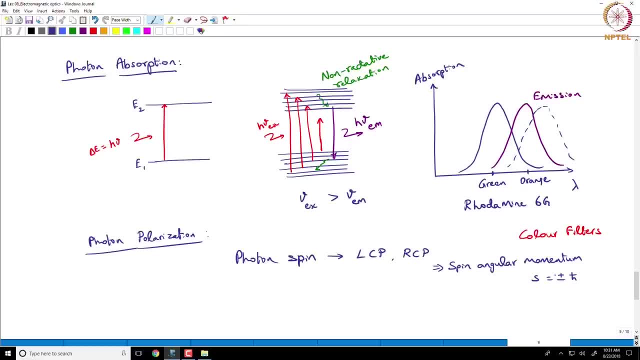 cross, right, So plus H cross for LCP and minus H cross for RCP. ok, So photon polarization can be quantified in a natural manner through this spin. you know the photon spin. Now you want to ask the question: what is linear polarization mean then? right, So the linear polarization. 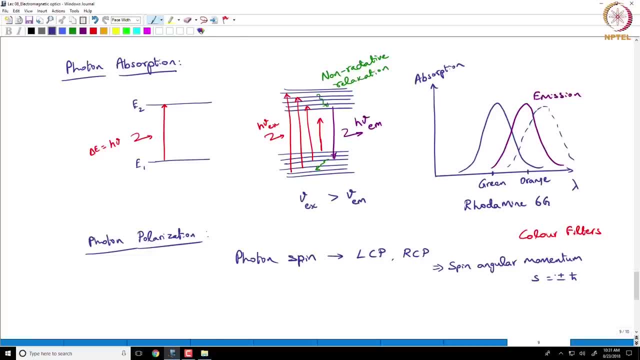 you can represent it as you know: certain particles that are collection of particles that are doing the left circular polarization and certain other particles that are doing the right circular polarization. Based on that mixture, you can define linear polarization. ok, So, since any polarization can be expressed in terms of right and left circular polarization, 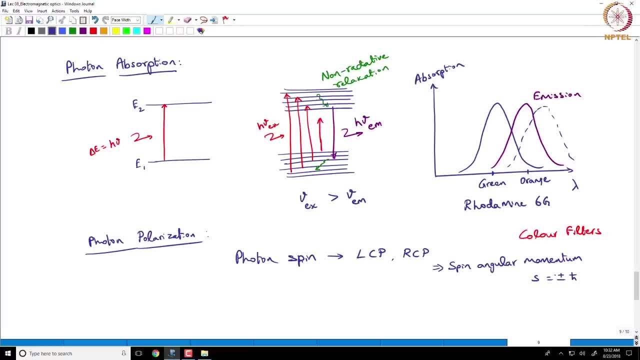 It is easy to say that you know, collection of these photons that are spinning one way, and, and, and, and photons that are spinning the other way, can be used to describe any other polarized state. ok, and reality, that is what it means as well. ok, So linear polarization is just in this case. 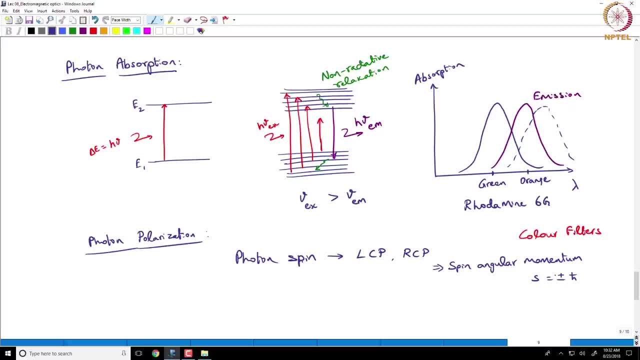 L Corona vodka总 telepathy o絡-CNN c-H nati-kit perché on¯ chat prefacehearer, ok, wa'qo, of left and right circularly fold rise photons. But the other intriguing part about this photon, 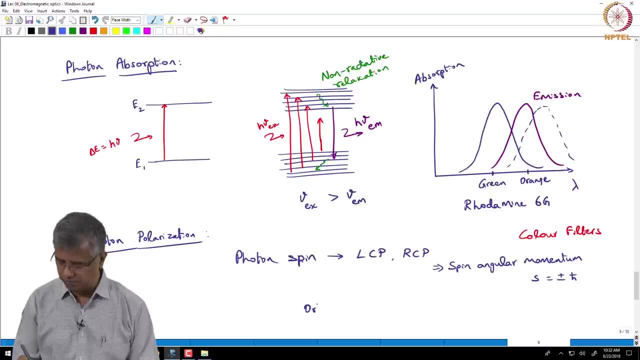 picture, is this concept of orbital angular momentum ok, So what does this correspond to? Orbital angular momentum corresponds to the fact that the photon can actually actually go in a sort of a helical path, as it is traveling, right, If it travels in a sort of helical path. 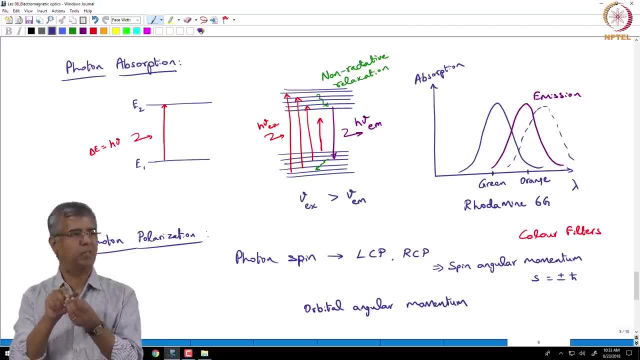 then it is. you have spin associated with that photon, and then there is also another momentum that it imparts its like. very simplistic example of this is that you want to put a negative constituent on one side and you want to put negative constituent on the other. 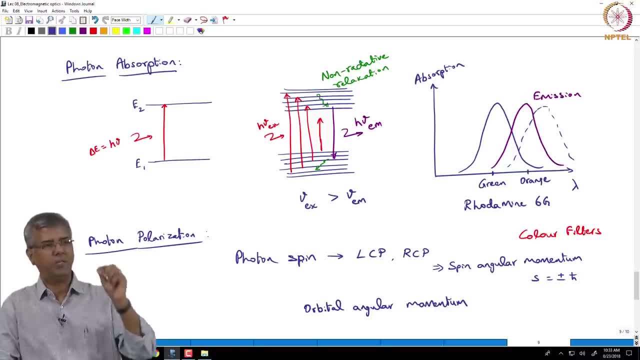 Pick a um, ransom it um, clouds the photon and then notify the electron in the sample controller. Right nail on the wall. right, You take a nail, hammer it through the wall. that is one way of doing it. The other way of doing it is you have a threaded nail and you impart a. 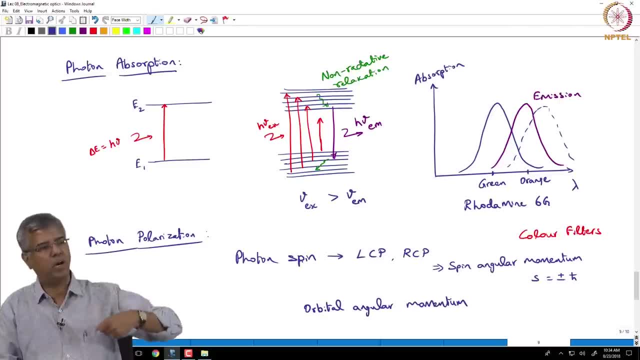 spin to that right. It is sort of a corkscrew motion, and through that you are able to go into the wall right. Which one is easier? The second one: why? Because you do have linear momentum and then on top of that you are imparting certain angular momentum. in this case, what? 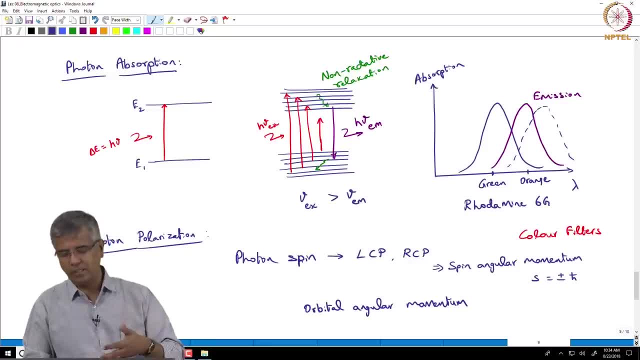 we are looking at it as orbital angular momentum. So these photons which have orbital angular momentum can actually carry a momentum which is defined, which is quantified as L, into h cross, where L corresponds to charge. ok, So you, basically L can be.